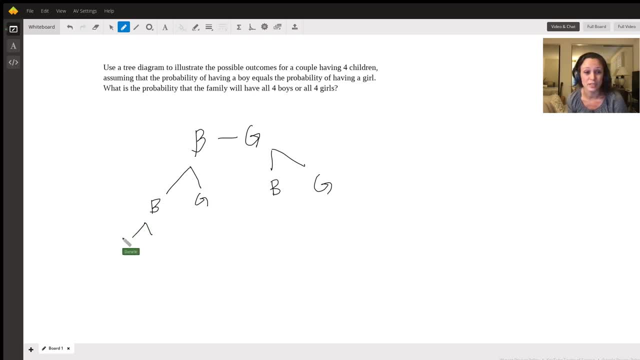 kid. now you see it's branching even more. If they had two boys, then they could either have another boy or they could have a girl. It's just like this. This is what the tree diagram looks like: B, G, B, G. 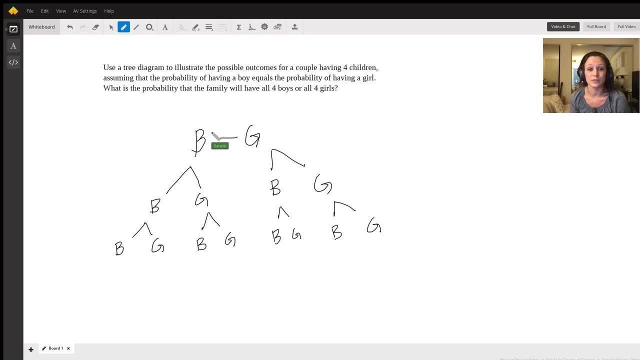 And then again. so this represents their first child, right here. Second child: the different options. Third child: different options. Now, fourth child: different options. They could either have a boy or a girl- Same thing. It's getting a little tedious here, but this is what. 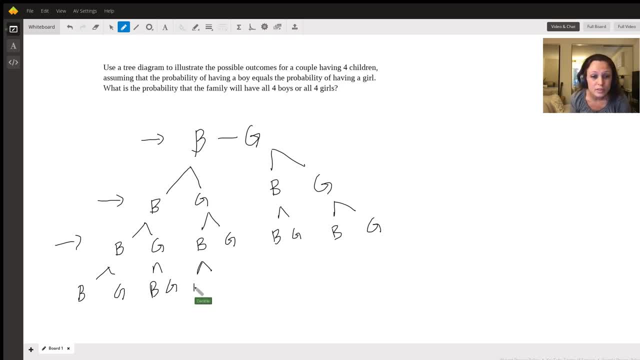 it's looking like Oops should write it in the same order. Just bear with me for a second Boy girl, boy, girl, boy girl. Okay, So now basically the options. the total number of possibilities there would be are represented by this bottom row, because this option here means: 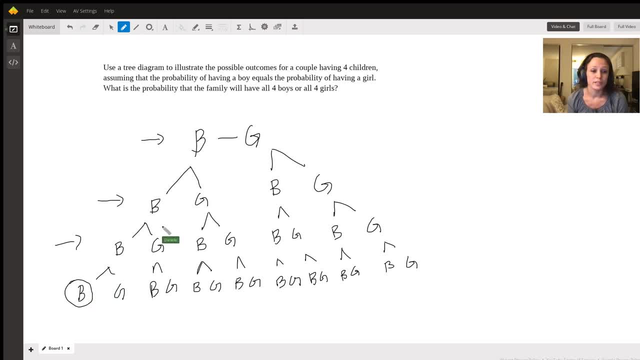 you've had boy boy, boy boy, So this option here means they had a boy boy, boy, boy boy. Now this option down here means they had boy boy, girl, boy and so on. So that means there's. 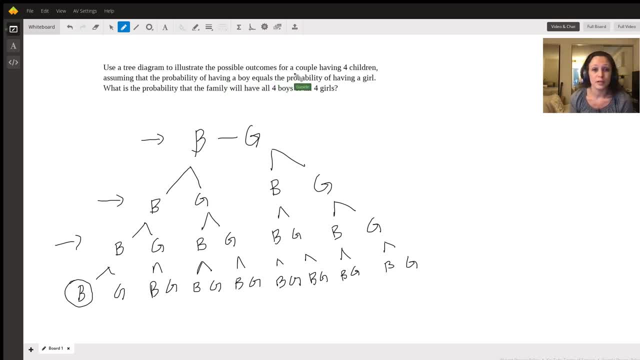 a total number of possibilities for the possible outcomes for a couple having four children. You know if order matters. if having a boy boy, girl boy is different from having a boy boy, boy girl, then the total number of possibilities are 1,, 2,, 3,, 4,, 5,, 6,, 7,, 8,, 9,, 10,. 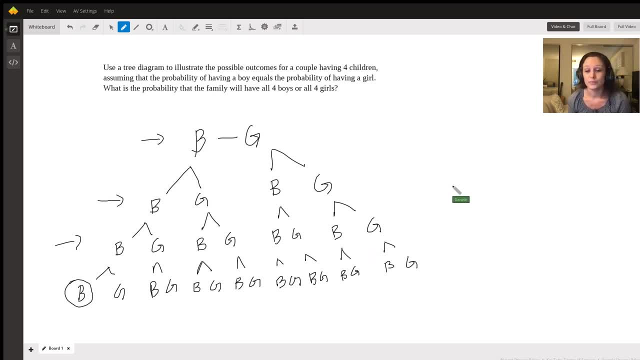 11,, 12,, 13,, 14,, 15,, 16.. So what they're interested in is having all four boys. There's only one place where we had all four boys. that was here. There's only one place where we had all four girls on our diagram, That's this. 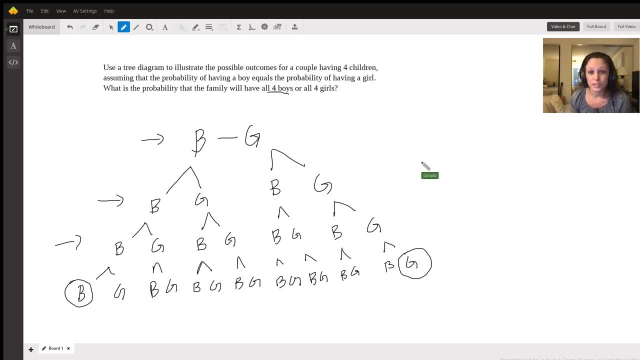 last option here. And then, of course, probability is equal to like the desired outcome over the total possibilities. In this case, we've got two of our desired outcomes, Which is all boys or all girls, the ones I circled here. So there's two And the total.